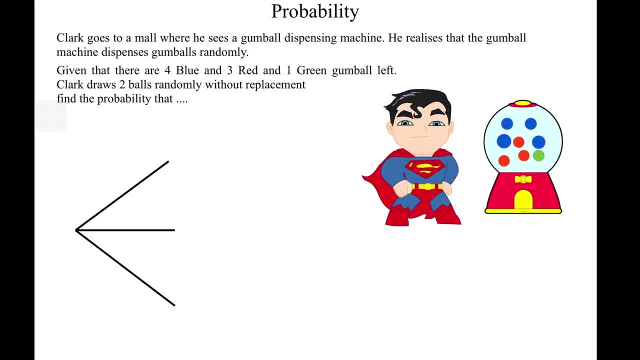 with three branches right, one for each color, so he could end up with a blue gumball, right, so let's give this wrong to blue. he could end up with a red one, right, so let's give this one red. or he could end up with a green one, so let's just give this one to green now, let's. 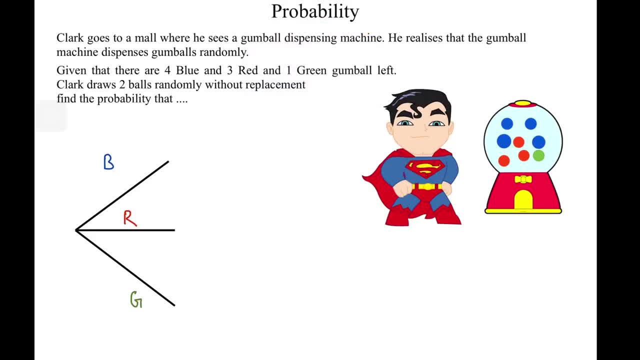 try and figure out the probability of ending up with a blue gumball. so for that we use the basic formula for probability, which is favorable upon total right. I'll just write it here in the corner. so the one formula that you need to know for probability is that it's equal to favorable outcomes upon 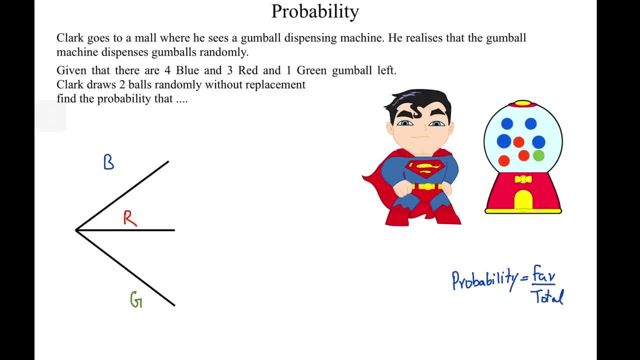 the total outcome. so if I'm talking about the probability of blue, I'm interested in finding out the number of blue gumballs and the total. so here I can see that the number of blue gumballs happen to be four and the number of total happened to be eight- all right, seven- and the number of total happens to 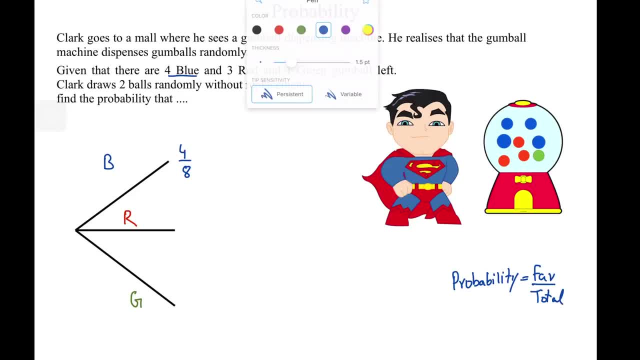 be eight, so that's taken care of. now let's talk about the probability of ending up with the red ones, so that we can see is equal to three over eight. and let's talk about the probability of ending up with the green one, so that we can see is one over eight, since we have one green and eight is the total now. I 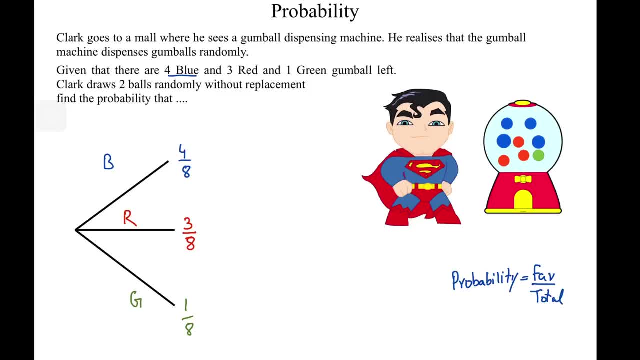 can see that the number of blue gumballs is equal to three over eight and the total is equal to three over eight. so that's taken care of. now let's take a look at the probability of ending up with a blue gumball. let's assume that he. 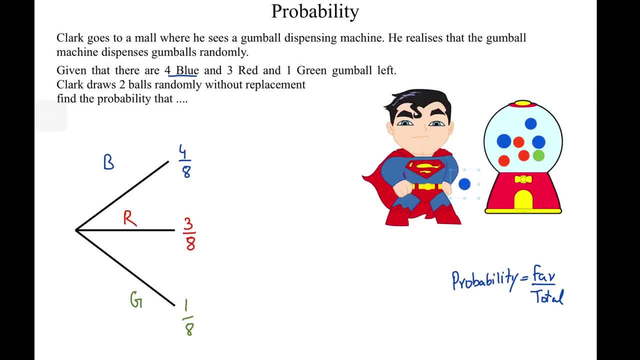 ends up in the first attempt. he ends up with a blue gumball in his hand. all right, so remember, we are under the assumption that the first gumball turns out to be blue. now, what does that mean? that means I'm gonna take a blue gumball. 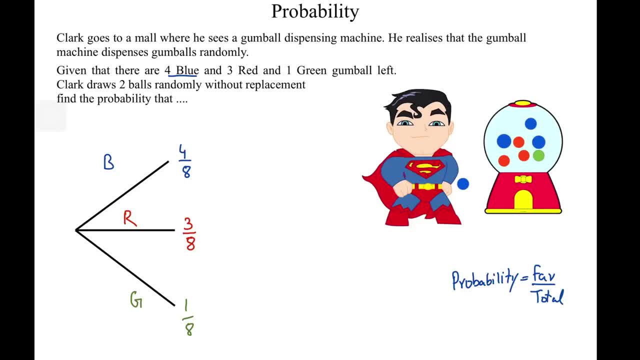 and I'm gonna put it in his hand, all right? well, I'm sure that I'll do so. now it's a second attempt. now again, we can see that in the second attempt there are three branches of blue gumballs in this example, so the first one is going to. 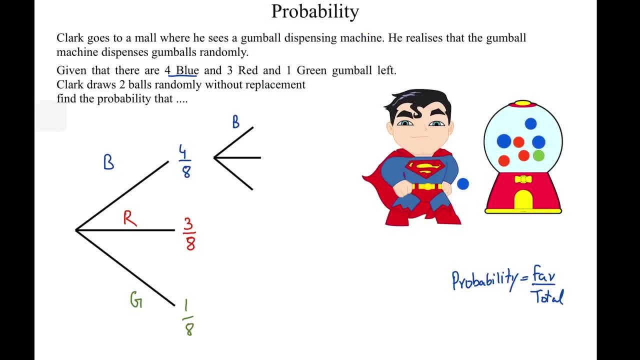 draw is gonna again have how many branches? three branches, yep, I'm pretty sure you got that right. so one for blue. but now let's see the probability of drawing a blue gumball. so we can see that the number of blue is not four anymore, it has gone down to three, and we can also see that the total is not eight. 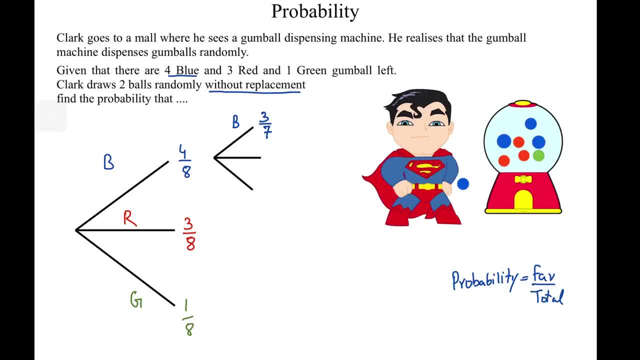 anymore. it has gone down to seven. right, because this is, this is without repeating. so now let's talk about red. so the number of red has remained the same, which is three, but the total, as we can see, has gone down by one. so that means the total is now seven, and it's pretty much the same case with green, the 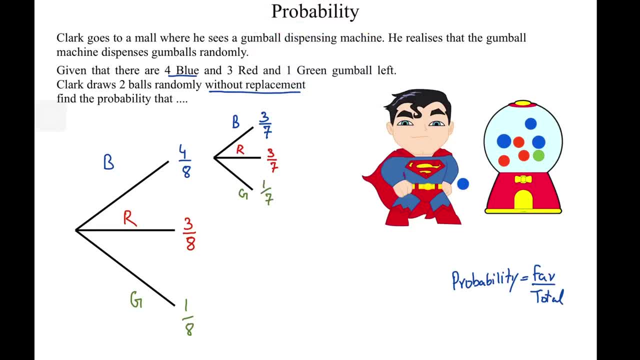 number of green has remained the same, but the total has gone down by one, so that's equal to one by seven. all right, so that was under the assumption that the first gumball turns out to be blue, but that may not be the case, all right, so what I'm going to do is I'm going to put this blue back to. 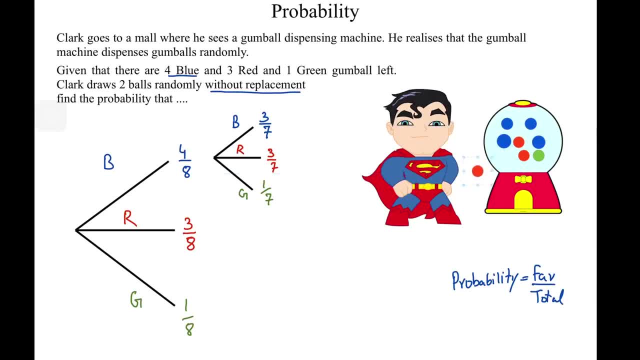 the machine, back inside the machine, and I'm going to assume that the first one to be red, right. so let's give clark a red combo, all right, i hope he's happy. so what i'm gonna do now is i'm gonna see that. fine, uh, the first one is red. so what are the number of colors that he? 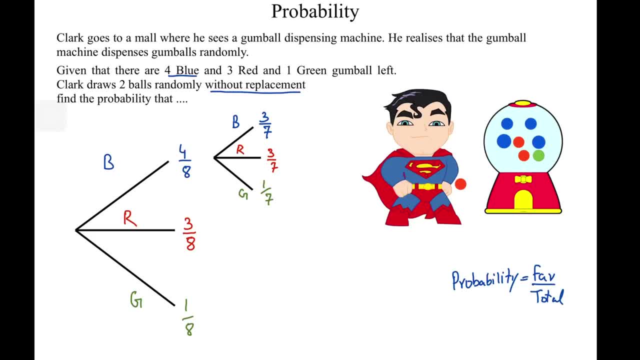 could end up with in the second attempt. so again, i can see that's equal to three. so what i'm gonna do is i'm gonna draw another tree. i hope i have enough space here, i think i do just squeeze it in. so here we have one branch per color. so this is for blue, right? so now let's see what's the. 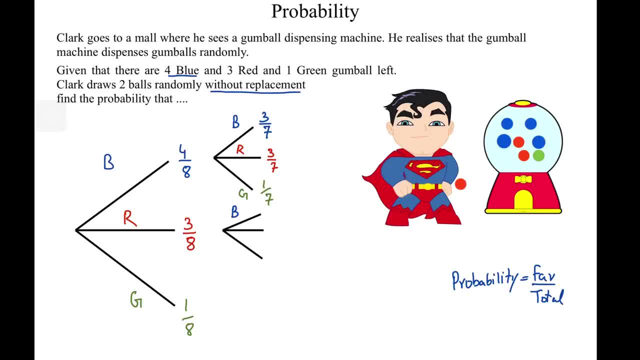 probability of drawing a blue gumball in the second attempt. all right, so we can see that the blue has remained the same, meaning it's four, but the total has gone down by one, so that's equal to seven. all right, i'm color coding it so that you guys don't get confused and let's see the. 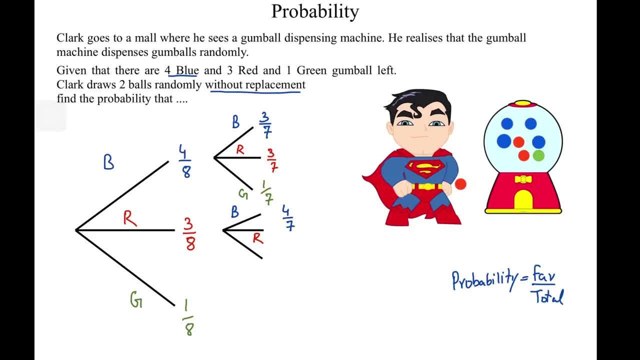 probability of drawing a red one. so we can see that the number of red gumballs are now two, since one is in his hand and the total has gone down by one. so that's equal to seven. all right, so by one. and let's talk about the green ones. so green, we can see, is one and the total, as we can. 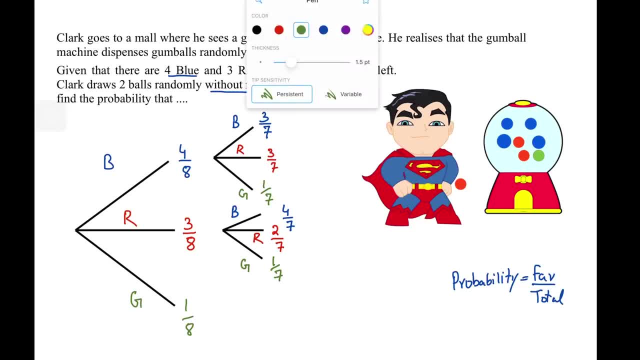 see, has gone down by one. so that's equal to one over seven. all right, okay, but that was again under the impression that this first one turns out to be red. but that may not be the case. why? because we also have a green one here. so what if he ends up with a green one in the first attempt? then let's. 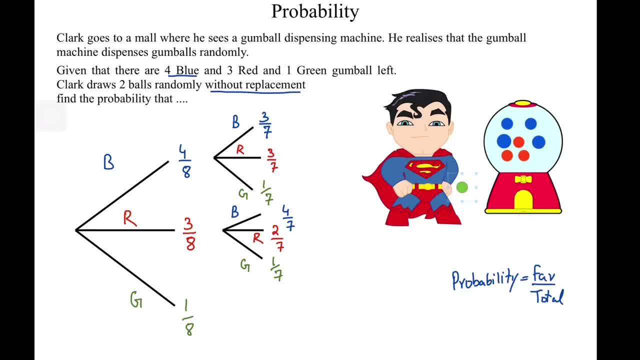 see what happens. so let's, let's give clark a green one now, if the first one turns out to be green. now you gotta be careful. you gotta be careful here why? because in the second attempt you can't have green anymore. because there were, there was.